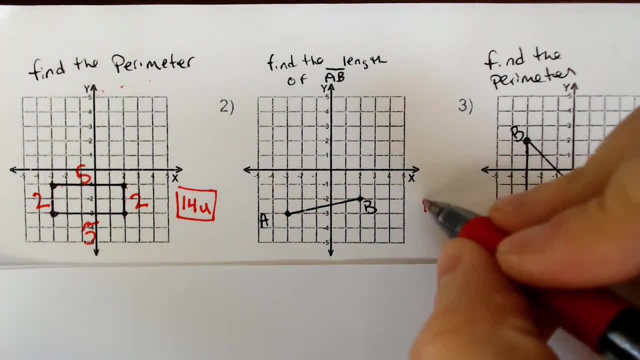 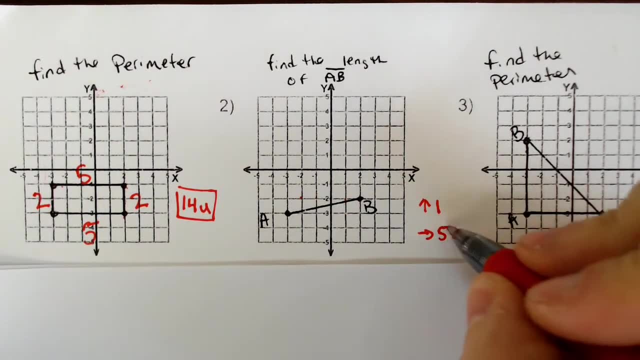 what is the slope? How much did I go up? Well, I went up by one and I went over by one, two, three, four, five. That is my a and my b for the Pythagorean theorem. So it's going to be one squared plus. 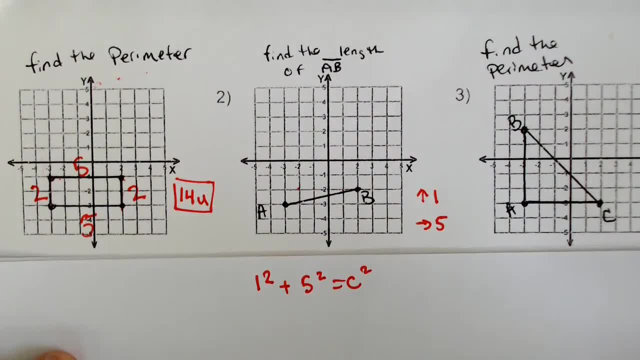 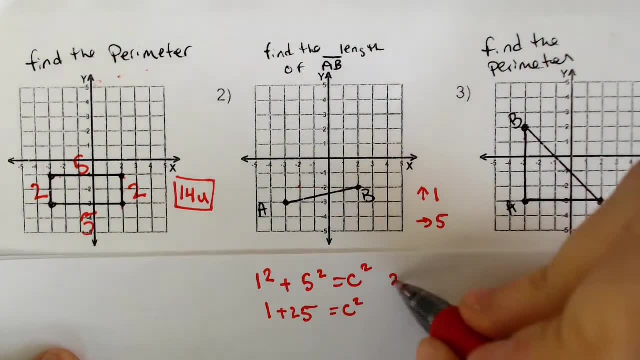 five squared equals c squared. and then we add one with twenty five and that equals c squared and you get twenty six is equal to c squared, and I want to keep this one as the square root of twenty six for c, Just like so. Okay, so we're going to have problems that. 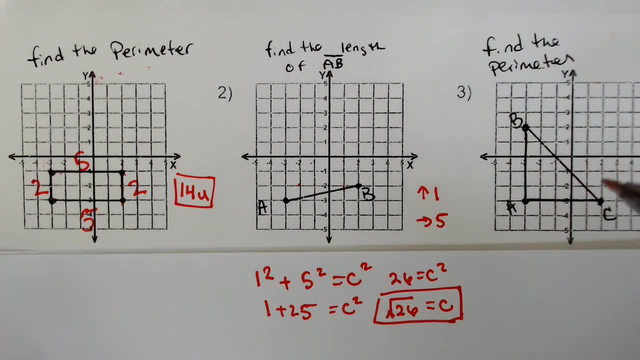 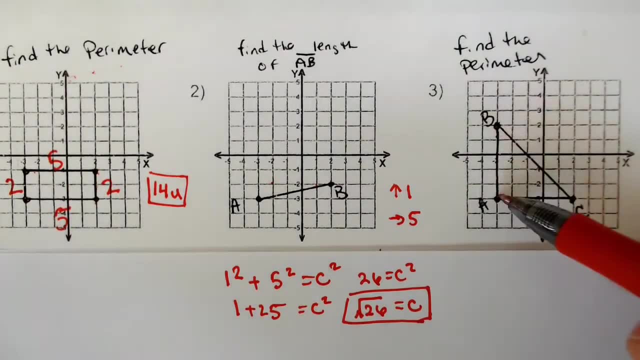 will require you to do that and find the perimeter of the other parts of it too. So that's going to be happening. on number three, If we look at this one, we can find the length of a, b and a c pretty easy. It went down by one, two, three, four, five and it went over by one, two, three, four, five. 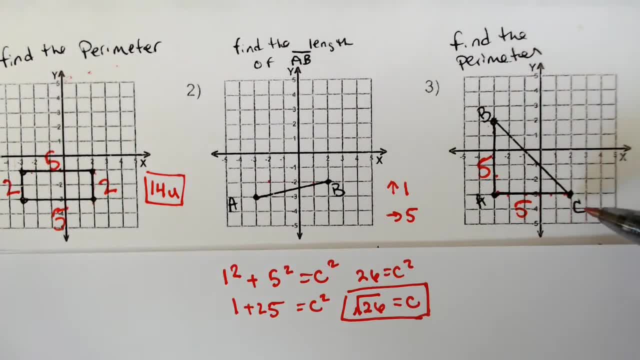 The dilemma is that we don't know what b, c is. Well, luckily, we just found the slope of this right triangle, and we got lucky that it was a right triangle too. So we know our a and our b for our Pythagorean theorem. So we got: five squared plus five squared equals c squared: Twenty five plus twenty five. 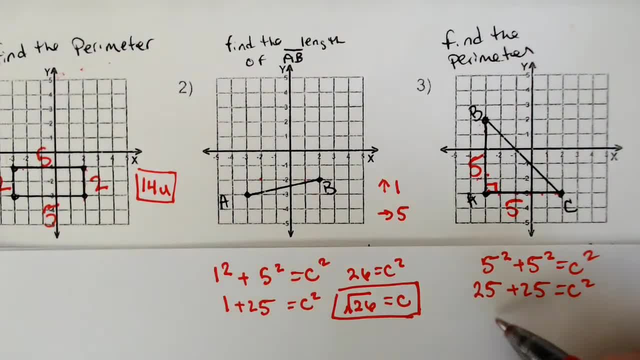 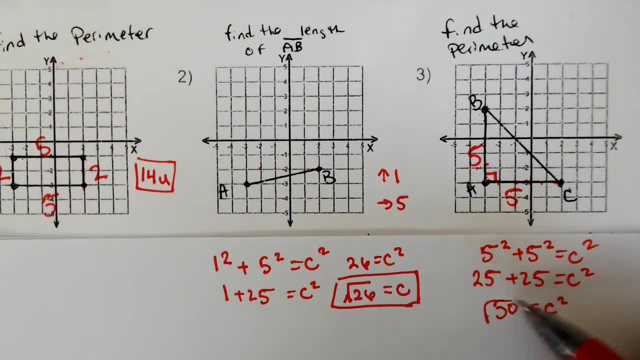 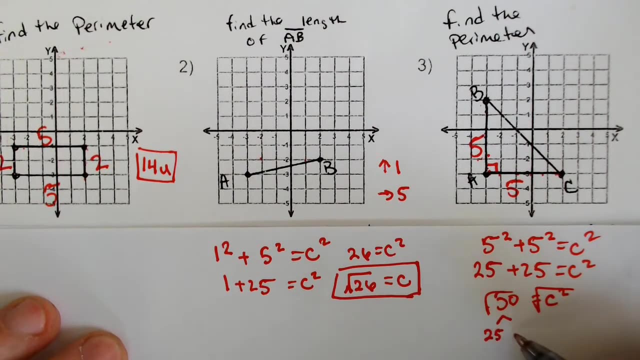 equals c squared, and then you get fifty. And in this case we are going to take that fifty and we are going to square root it And we get: if you simplify the fifty, it would really be twenty five times two And the square root of twenty five is five. so this is five times the square root. 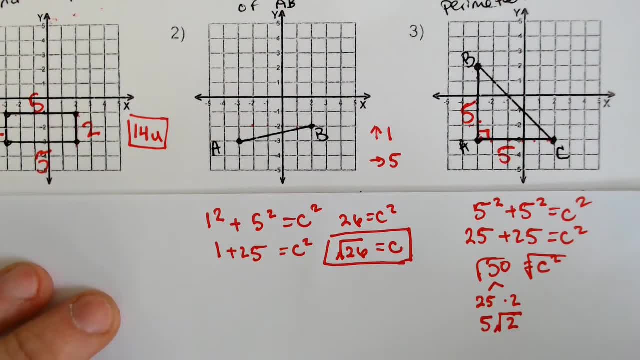 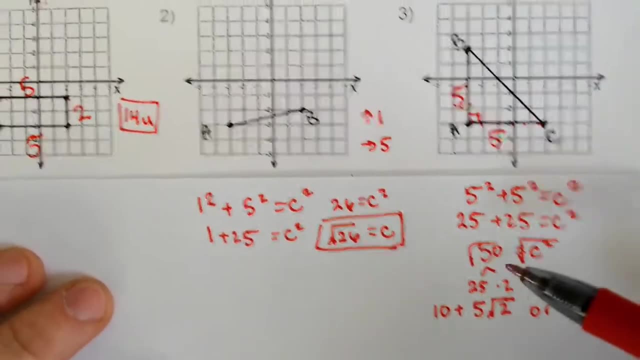 of two, And you could write this answer in one of two different ways. You could write it as the five plus five plus this, which would be five plus 5,, 10 plus 5, square root of 2, or you could find the decimal of what the square. 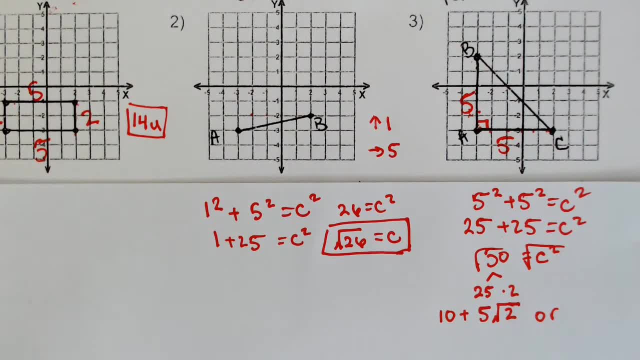 root of 50 is, and if you do that, then you are going to be able to get a decimal answer which is approximating what it actually is. and the square root of 50 is 7.07.. If we added that to the 5 and the other 5, we would get the full perimeter. so that would. 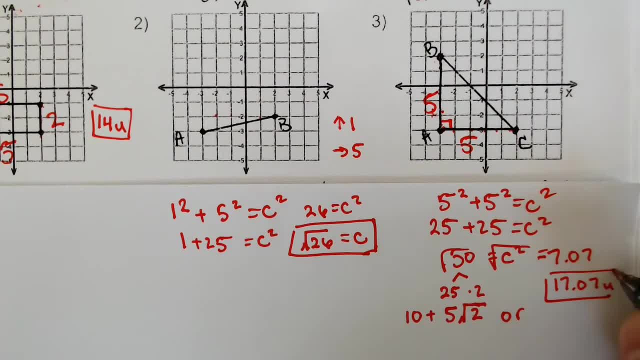 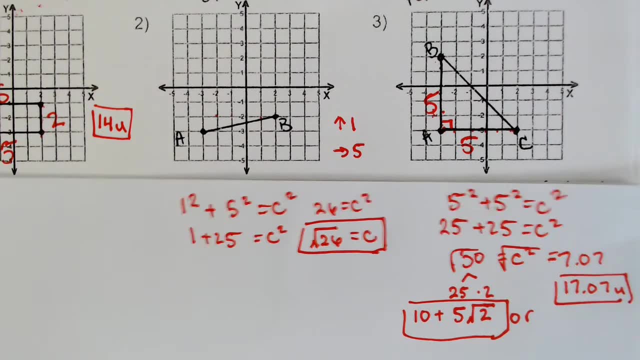 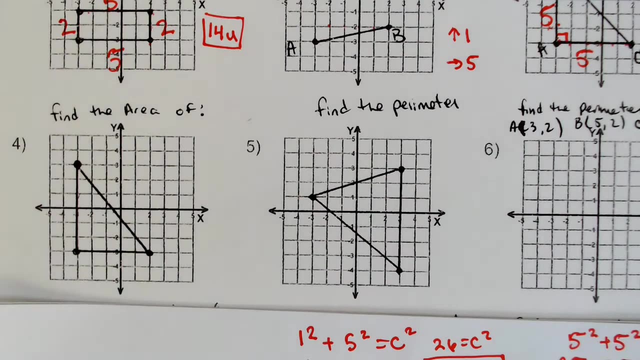 be 17.07 units, or you could use the more specific answer of 10 plus 5, square root of 2.. Moving right along problems may also require that we find the area, and in order to do that, we are going to need to know what is the area formula for a triangle. 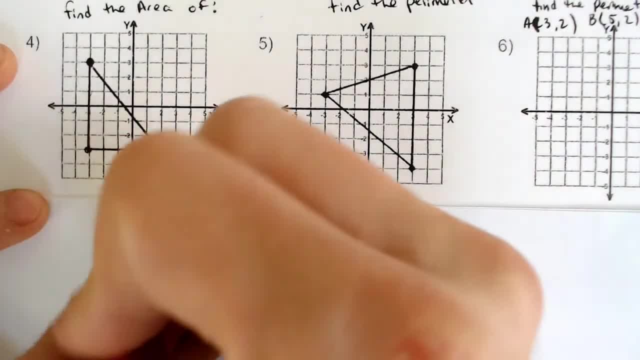 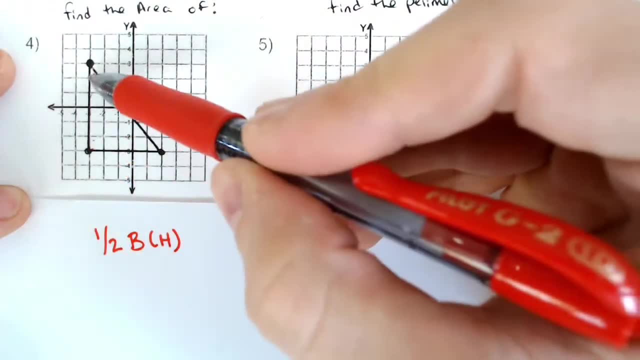 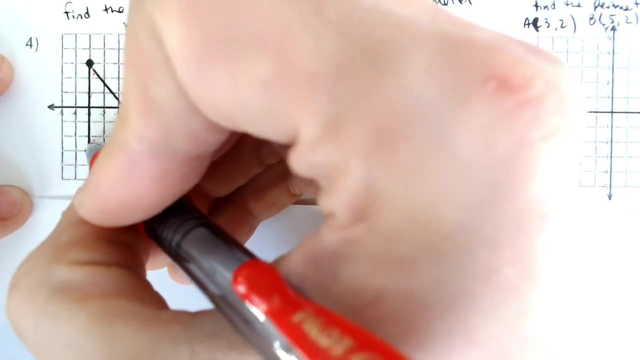 Well, the area formula for a triangle is 1: half the base times the height and the height is: is this part up and down and the base is the bottom of the triangle and hopefully it will be a right triangle, because if it is not a right triangle, one of those two 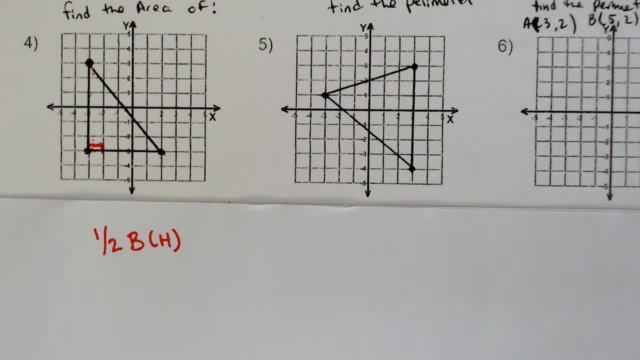 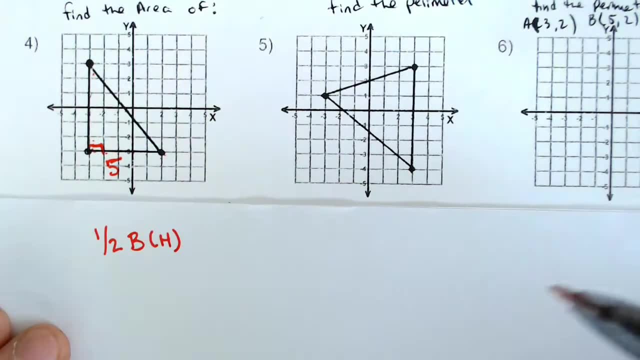 things may be difficult to figure out, So let's start with: what is the base? 1,, 2,, 3,, 4, 5.. What is the height? 1,, 2,, 3,, 4,, 5,, 6.. 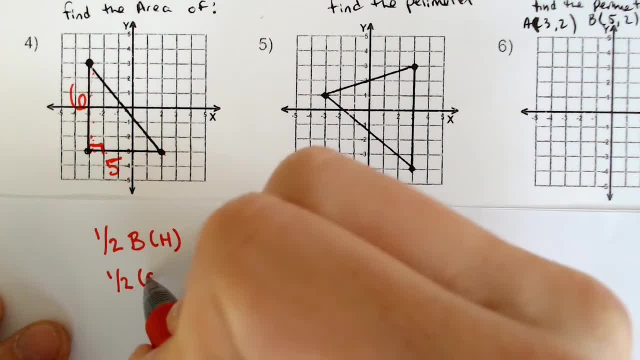 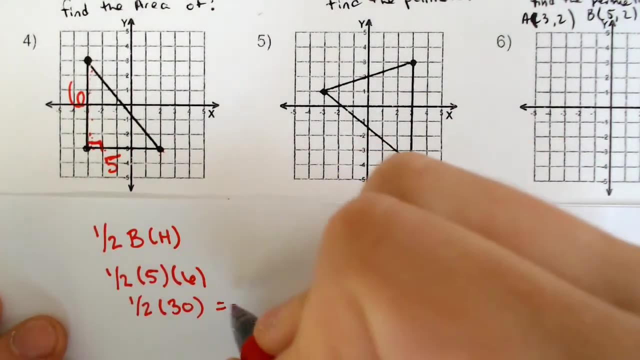 So we just plug it into the formula: 1 half base times height. My recommendation is to multiply the base and height first, and you end up with 1 half times 30,, which is just half of 30, or 30 divided by 2,, and that gets us 15, and it's. 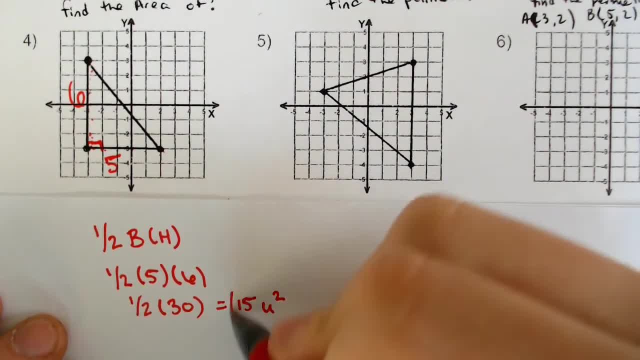 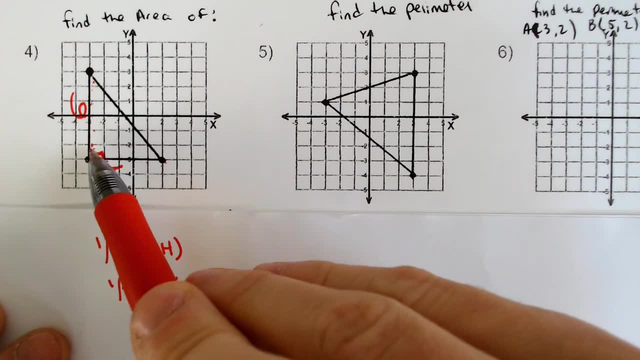 not going to be 15 units, it's going to be units squared, because area is in units squared, not just units. And if that, What that means is if we were to add up every single one of these squares: 1,, 2,, 3,, 4,, 5,. 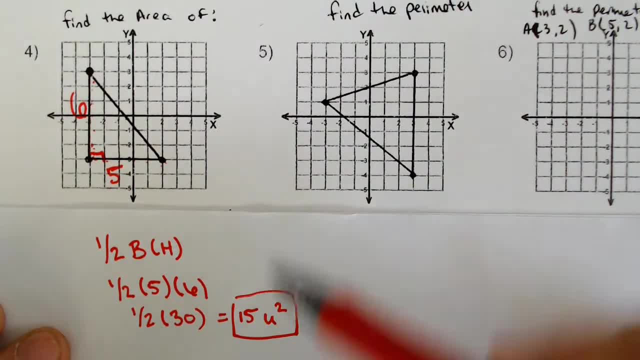 6,, 7,, 8,, 9,, 10,, 11,. we would get 15 of them in there, and some of them would be part of a square and another part of a square, but they would all add to equal 15 units squared. 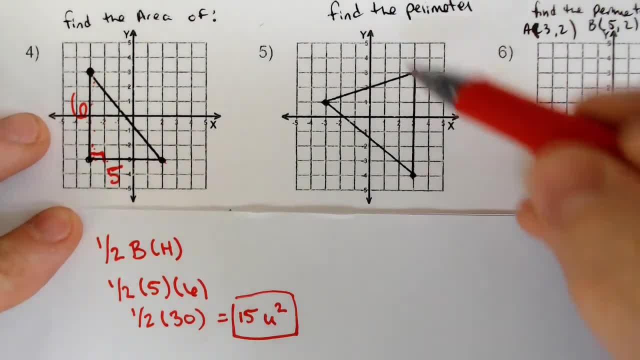 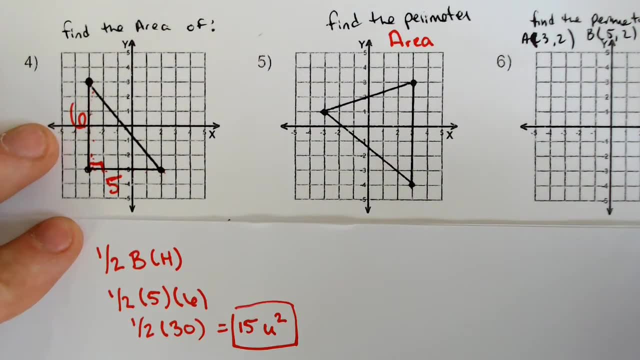 Okay, So this next problem. it says find the perimeter, but I'm also going to find the area, and I'm going to start with the easier one of the two, which is actually the area. For the area of this problem, We are going to need to figure out the base and the height, and any side can be the base. 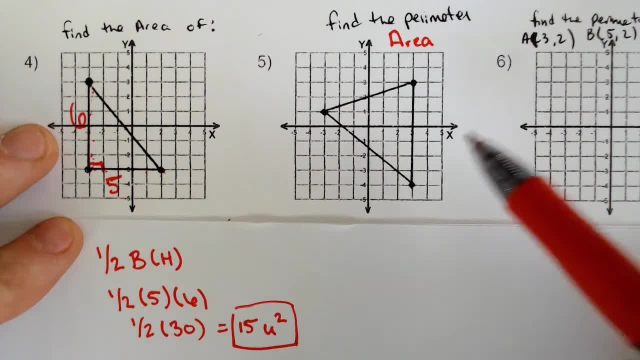 or the height. but you need to be very careful on how you make your selection and you need to be more so careful on how you choose what is going to be the base of your triangle. You would prefer, highly prefer, that the base of your triangle go straight up and down. 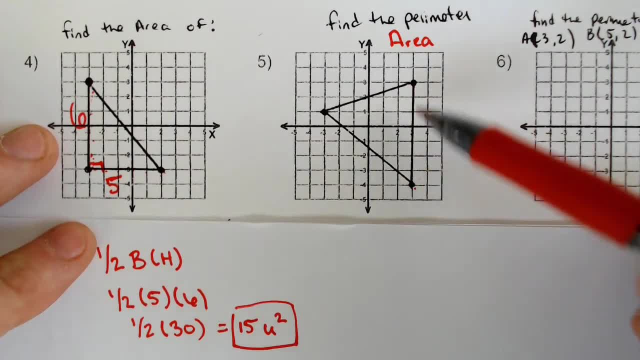 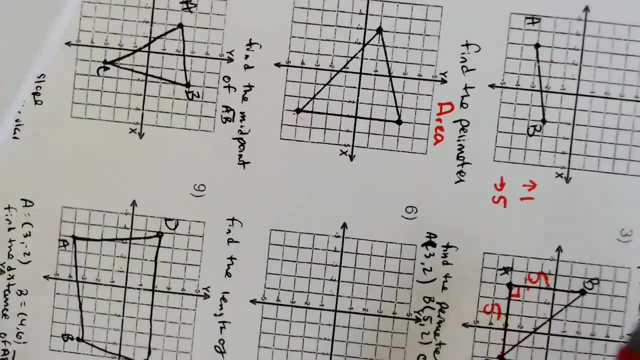 or straight, left and right, and in this case we have this one right here. That is what I'm going to call the base of this triangle. If I were to turn it like so, then I would be able to figure out what the base is, and 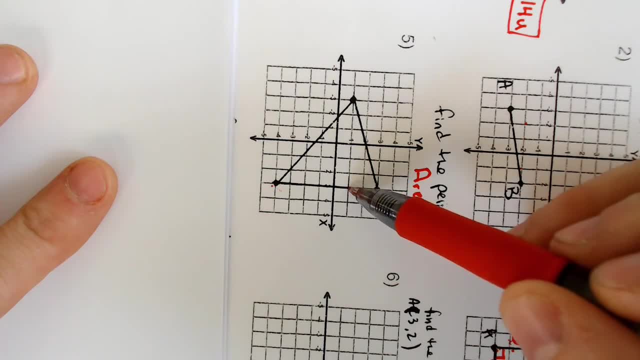 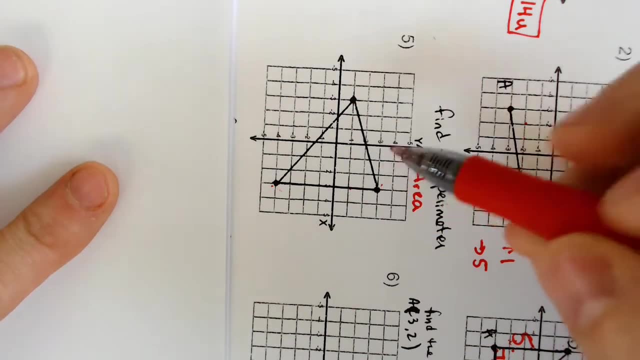 it would look like the bottom and the height is which. the height is not the line, but how far does it go? straight up to the opposite vertice, and in this case it goes up by one, two, three, four, five, six. 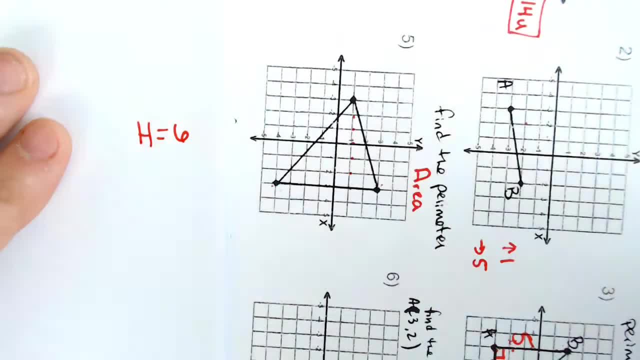 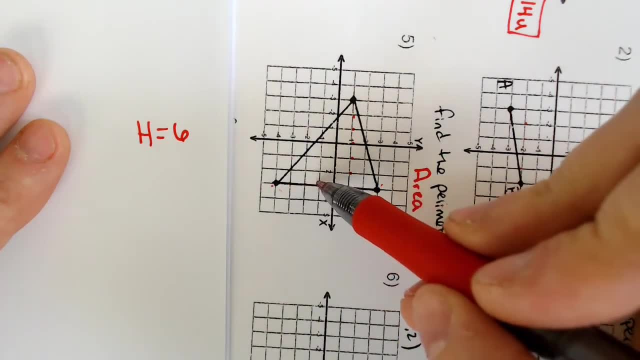 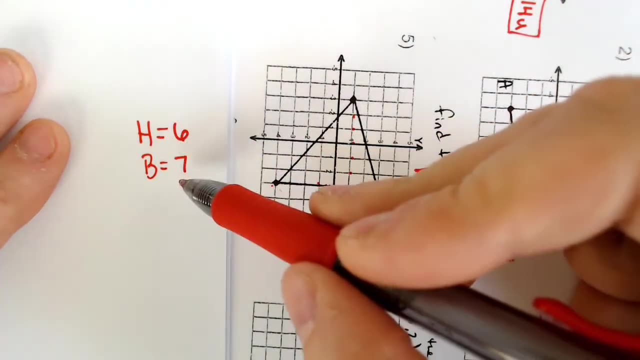 So that means that my height is six. My base is the bottom, Which was really kind of the side of the triangle at first- is one, two, three, four, five, six, seven. So we have our base and our height. 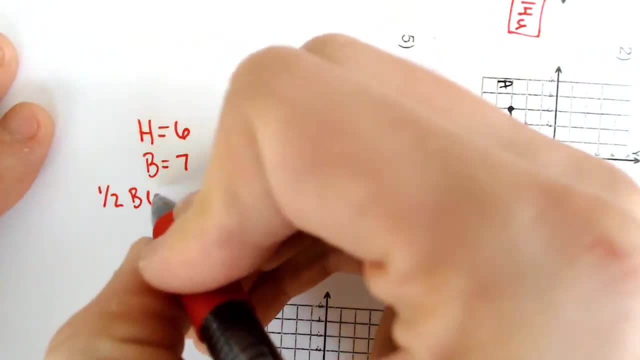 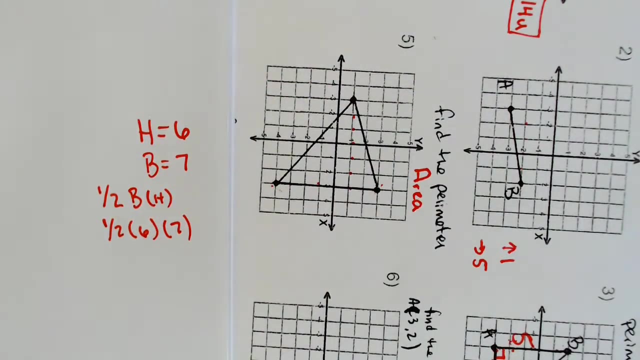 We have to plug it into the one half base times height formula and again, it's way easier if you take one half the base and the height and multiply those two first, because occasionally it just works out better that way, and in this case it's no different. 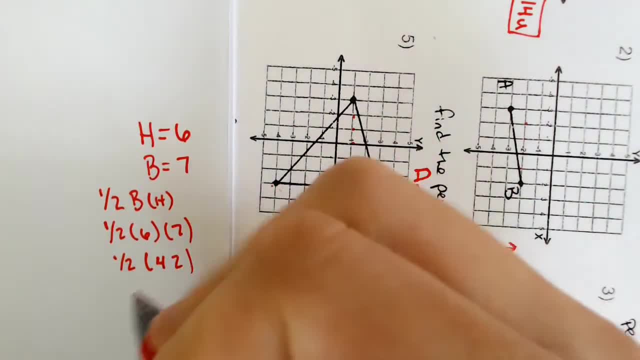 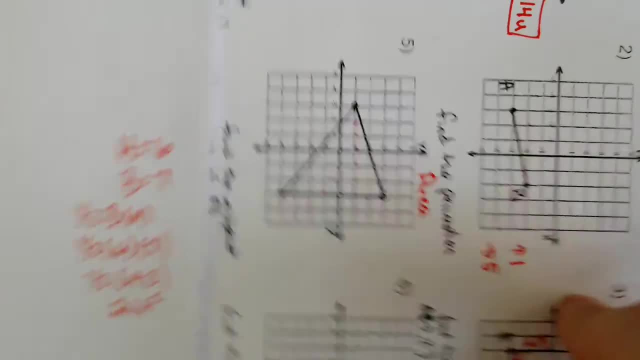 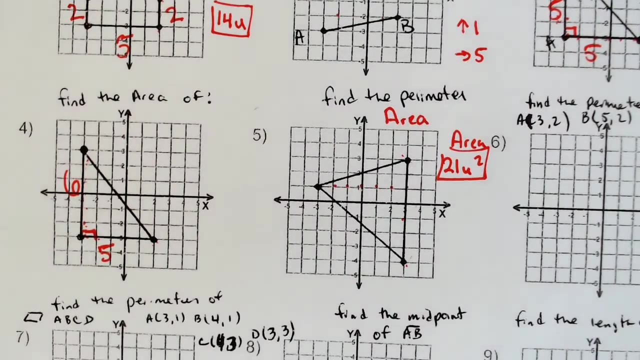 We get one half of forty-two. Half forty-two is forty-two divided by two, which is twenty-one units squared. okay, So that means that the area of this triangle is twenty-one units squared. That's the area. We're now going to find out what is the perimeter. 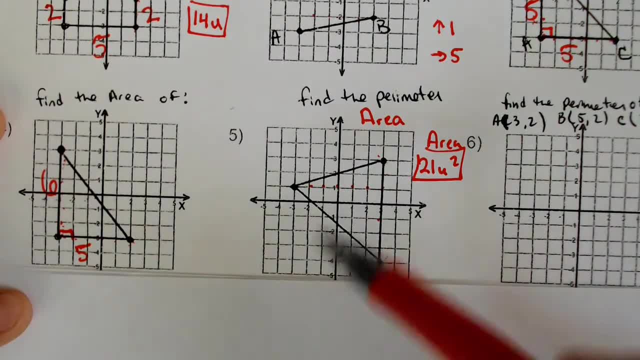 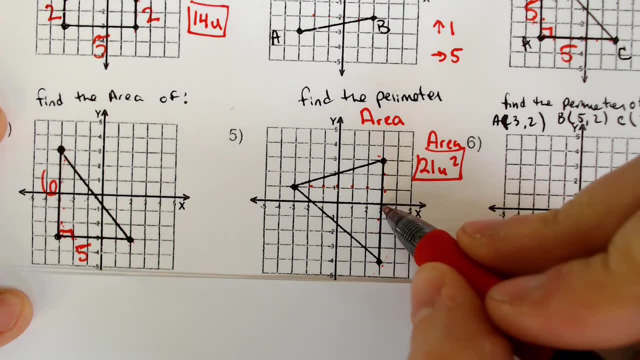 The perimeter is going to take a bit more time because the perimeter needs to add up all three sides. So far, the only side I know is this one right here. That is one, two, three, four, five, six, seven. 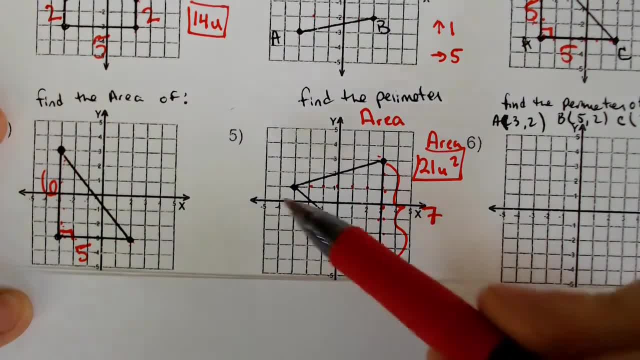 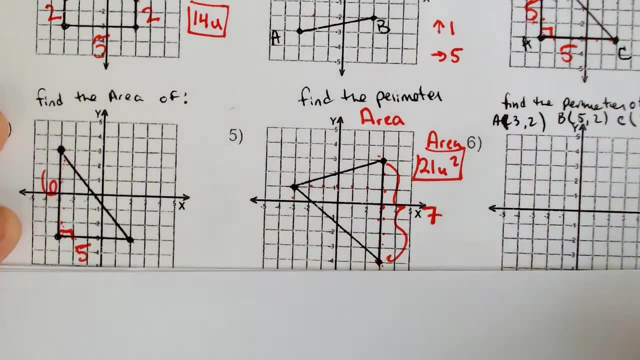 So that part's seven. but I still need to figure out what is the length of this side and what is the length of the other side, and I'm going to do that by just counting the slope for both of them to get my A, B and C for the Pythagorean Theorem. 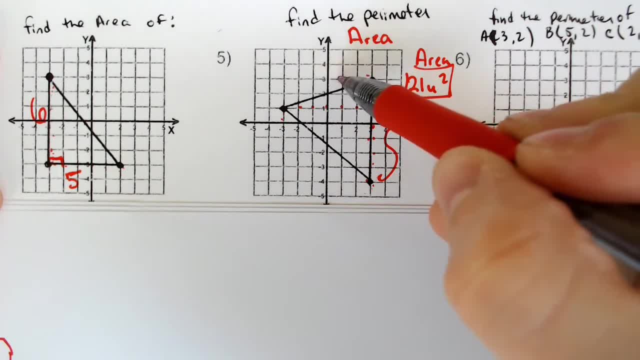 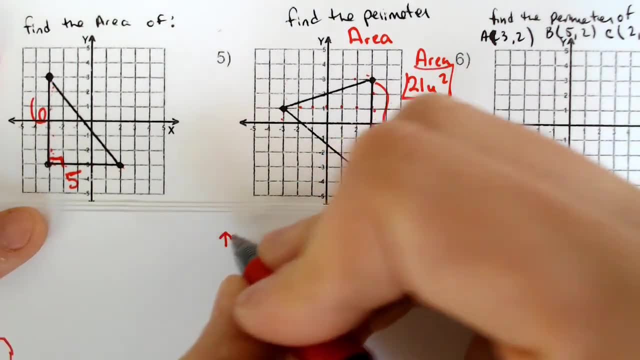 So I went up by one, two and over by one, two, three, four, five, six. Let's count it again: Up by one, two, over by one, two, three, four, five, six. So up by two. 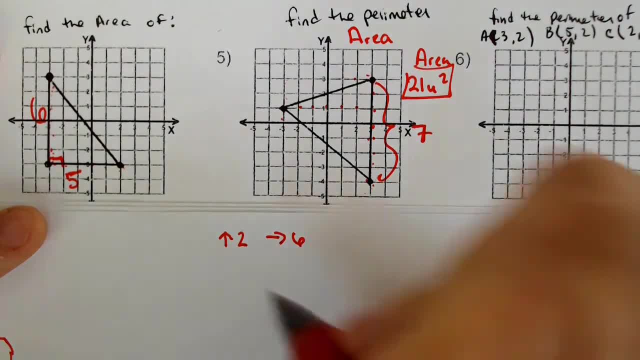 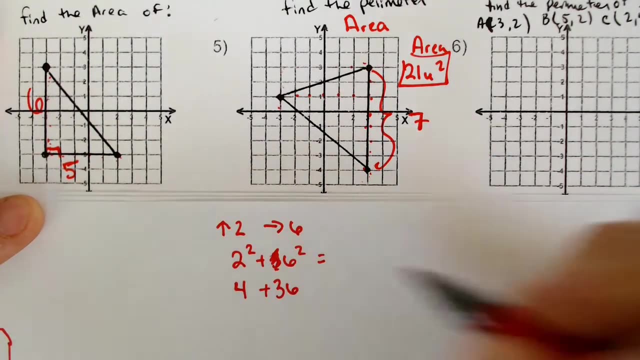 Up by two Over by six. My A and my B are two and six. I add them together. I don't know why I wrote thirty-six. I already squared it. So two squared is four and six squared is thirty-six. 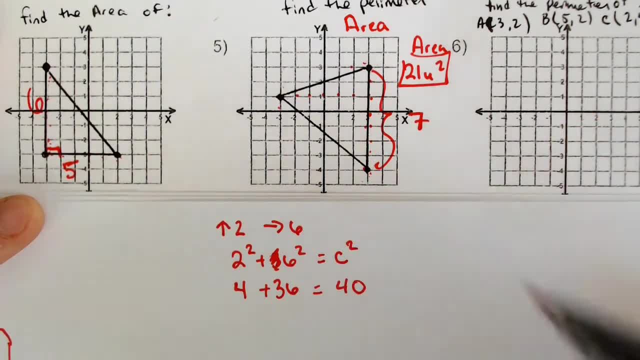 We add them, we get forty. And remember that this is the C squared. so if that's the C squared you just square root that number. The square root of forty as a decimal Is forty. forty square root six point three, two. 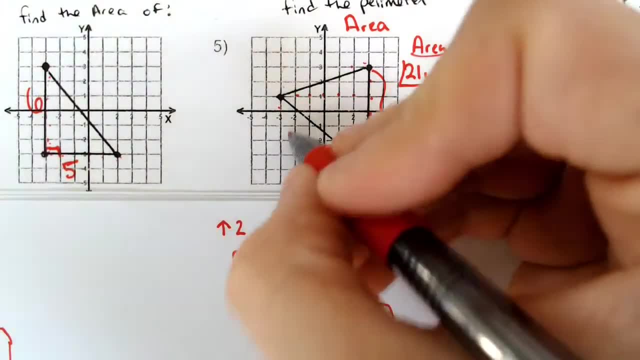 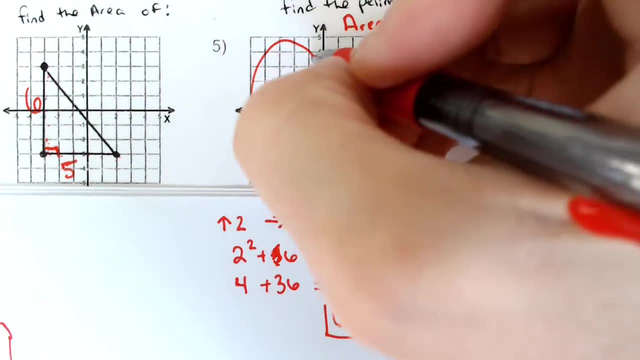 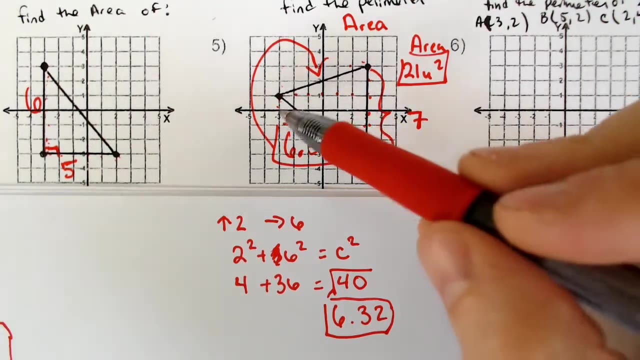 Okay, So that means that that side right there is six point three, two. We now- oh, I lied, is this side right here My mistake? So we still have to find the length of this bottom side, which I just incorrectly labeled. 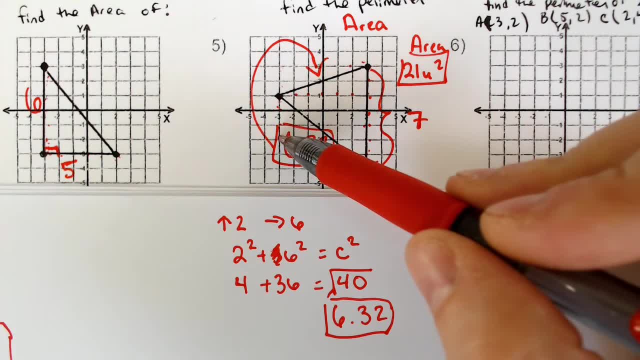 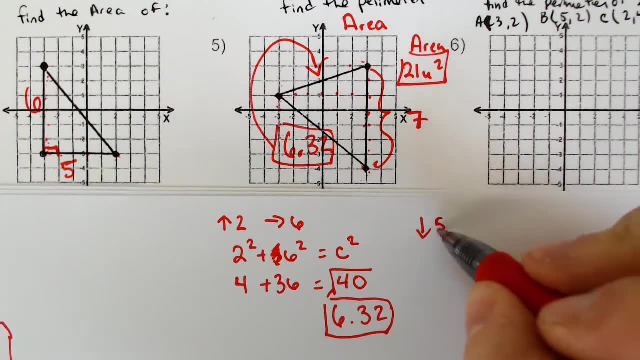 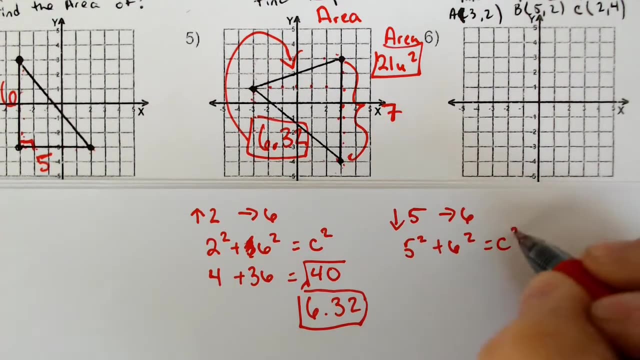 Which is going to be again. count the slope: One, two, three, four, five and over by one, two, three, four, five, six. So it went down by five and to the right by six. That is your A and your B. five squared, six squared equal C squared. 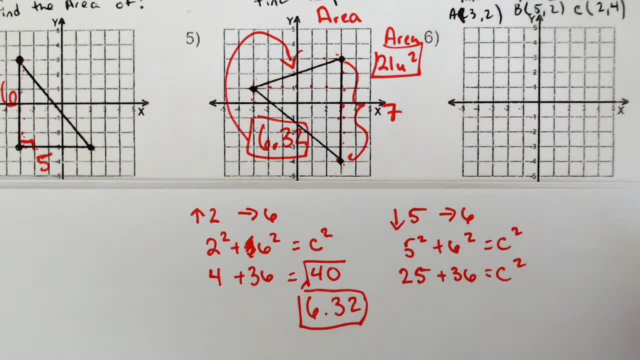 Twenty five plus thirty six equals C squared. Add them together and we get twenty-five plus thirty-six is sixty-one, So sixty-one is equal to thirty- một. That's right. Sixty-one 65.. Sixty-one, Sixty-one. 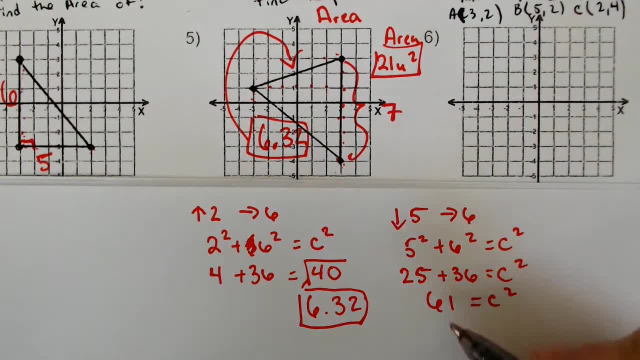 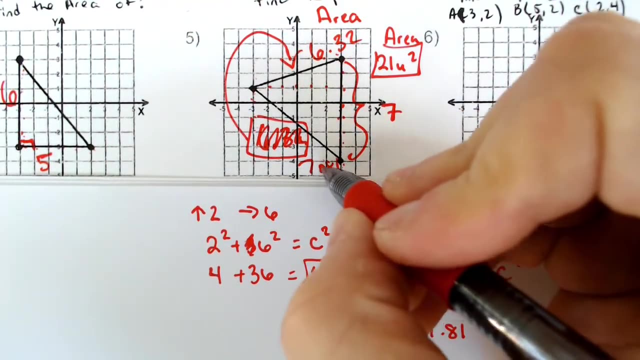 Sixty-one Sixty-one c squared, the square root of 61 gets us our answer, and that is 7.81. so this side is 6.32, but this side down here is the 7.81, and if we want to find the perimeter, all we have to do. 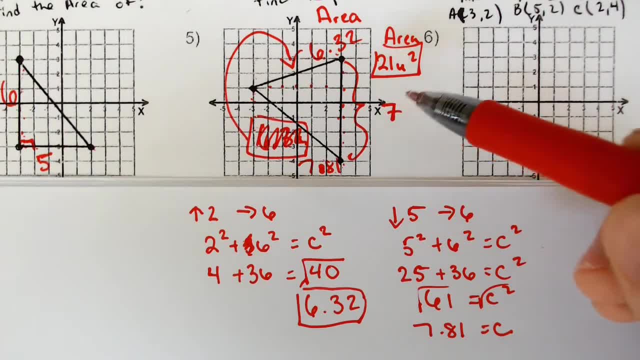 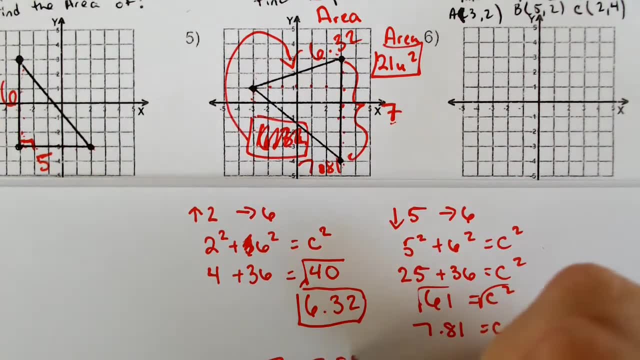 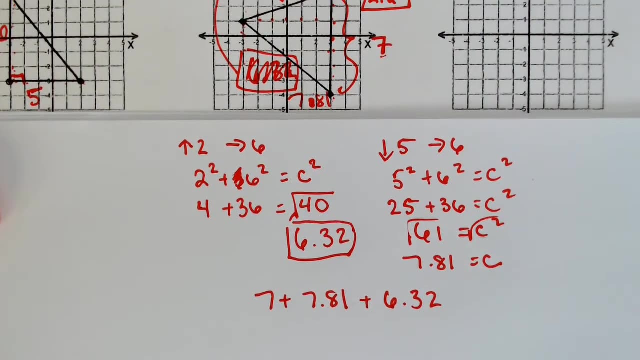 is: add up all the sides. so we already have all three sides. we just have to add them up. that is going to give us 7 plus the original 7 going around clockwise, 7.81 and 6.32. if we add up those three sides then we get our full perimeter and if i do that, 6.32.